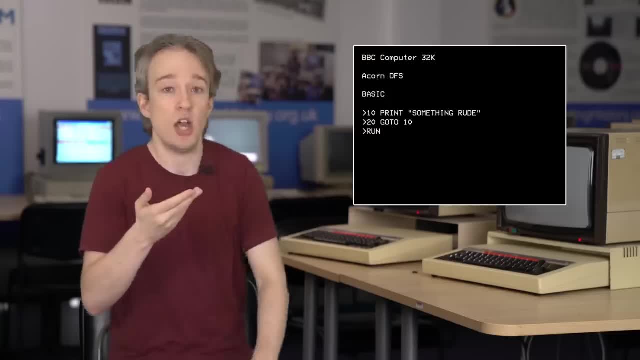 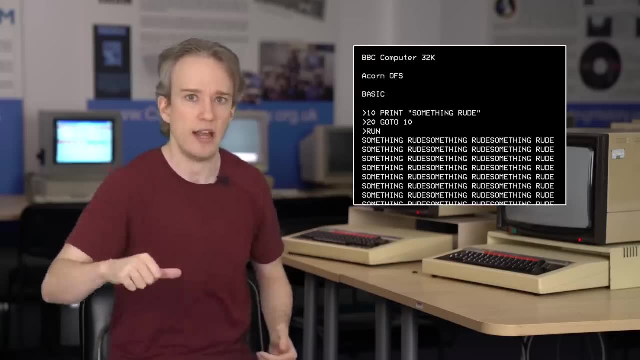 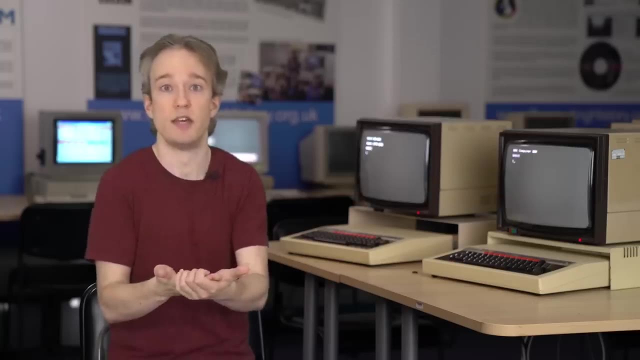 type in something like this And suddenly your display model was endlessly typing out something rude, until you hit the break key or turned the computer off and on again. That is a really simple example of a program that will never halt- And it is deliberately written that way, But programs that never halt. 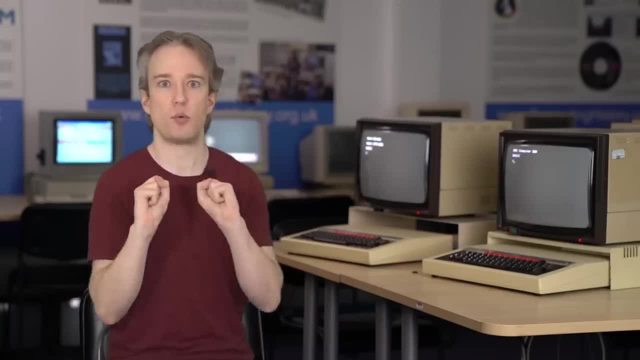 can also be written accidentally. We've all had that moment where something we're working on freezes stuck in an endless loop, doing… something, And you have that horrible moment of trying to remember whether you saved recently or not. It would be brilliant to be able to analyse. 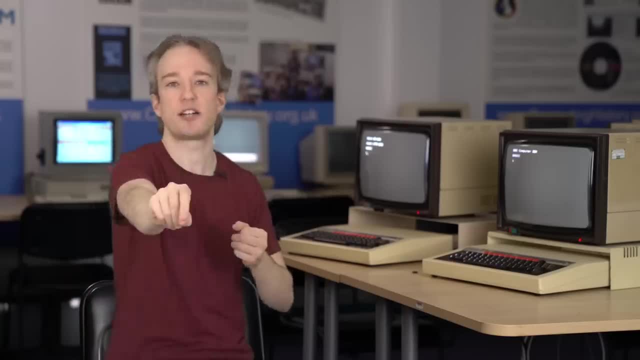 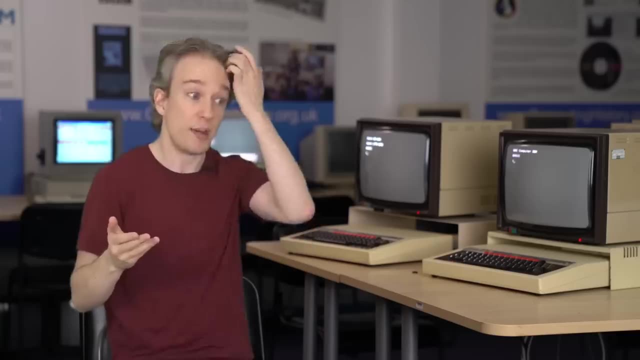 code any code and say definitively yes, eventually it'll halt, or no? there's a point in there where it'll keep looping forever. if this happens, Which sounds like a simple problem, It's actually impossible, Literally, mathematically impossible. and how we found that out? 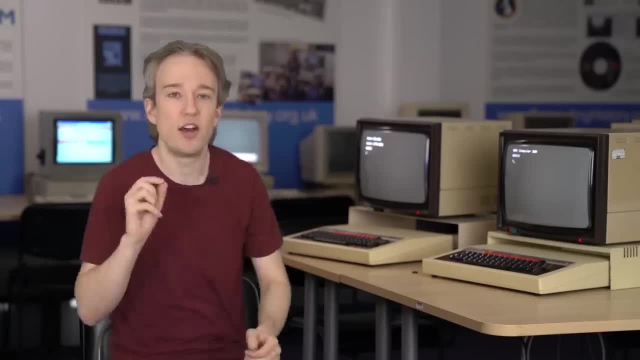 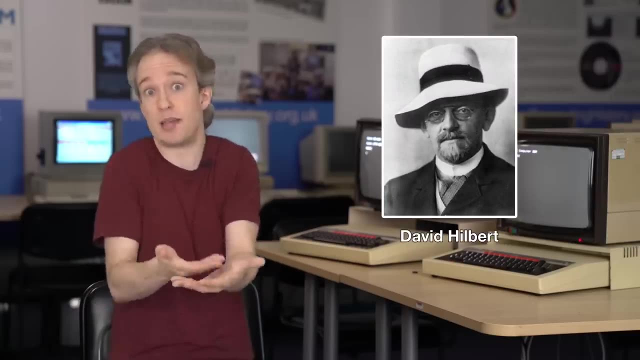 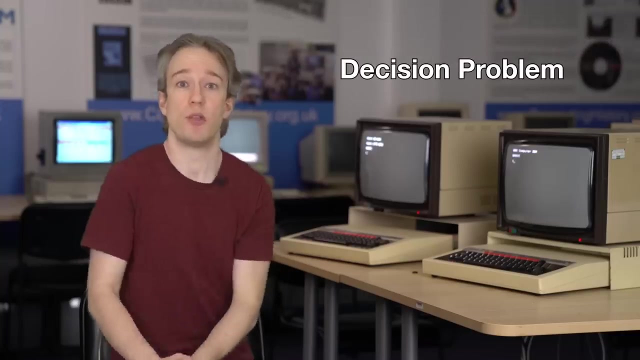 comes from before electronic computers were even invented. In the early 20th century, a mathematician named David Hilbert posed a series of problems that he thought mathematics should be able to answer. One of them came to be known as the… the, uh, the decision problem, which is, in short: can we determine if any given statement? 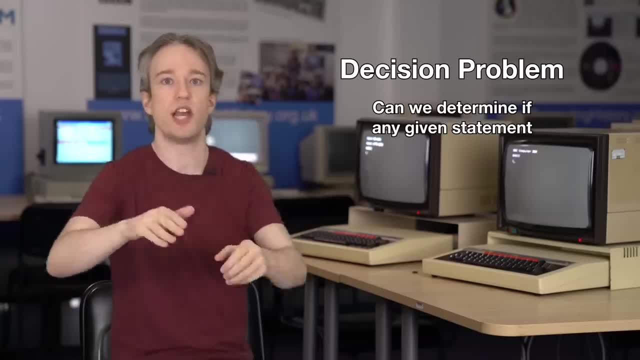 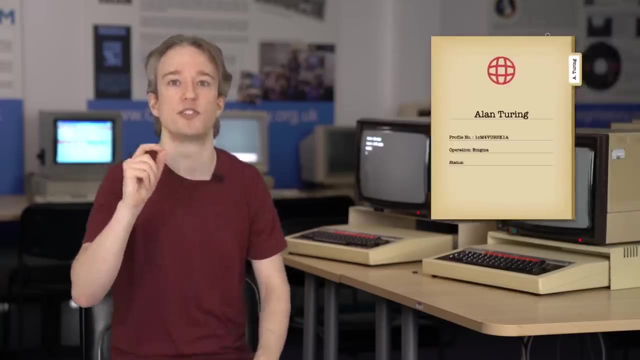 meaning absolutely any logical statement or problem in the universe is provable or non-provable. Given enough time, could we find an answer to everything. Hilbert was optimistic that the answer would be yes. Other mathematicians proved him wrong. One of those mathematicians was Alan Turing, and to explain his proof: 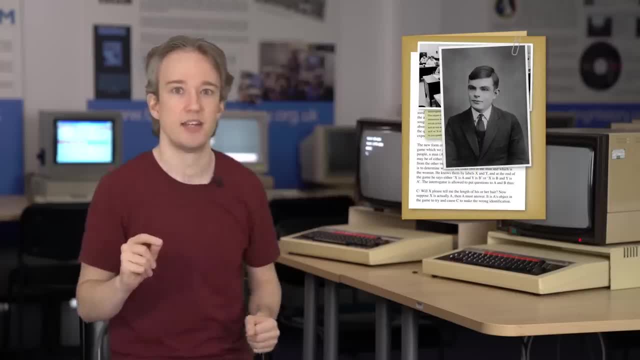 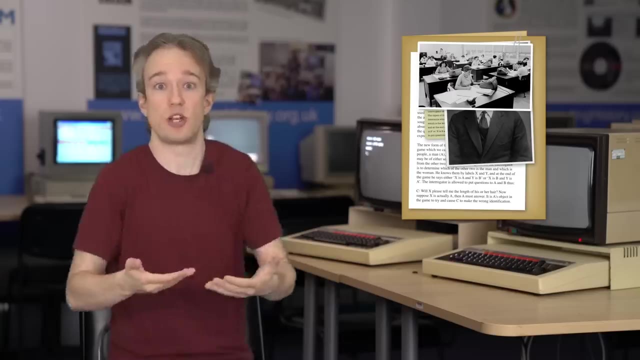 we first need to look at the tool that he used to make it. Turing was looking at the mechanization of logic and computation. A computer at this point wasn't an electronic thing. It was a job description: People who sat in rooms doing calculations over and over and over. They were called computers because they computed. 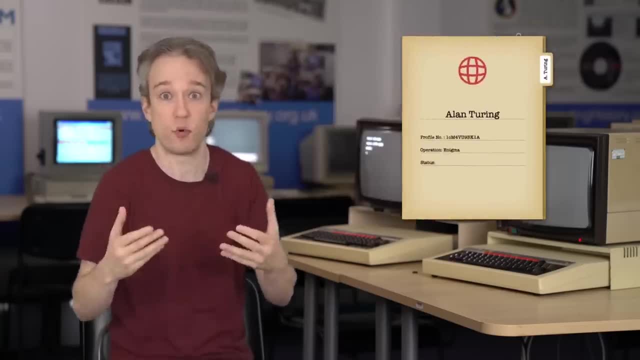 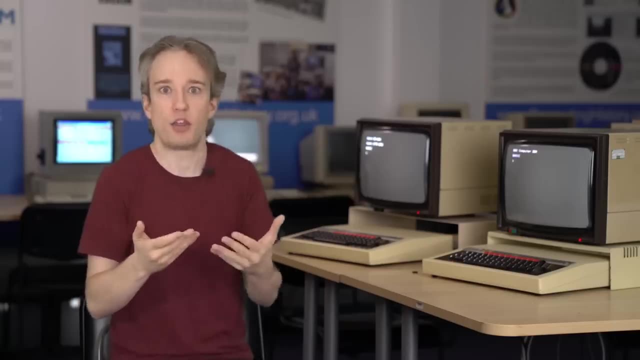 Turing was fascinated by the idea of automating that process. The dream was if everything could be encoded into numbers and if we had mechanical methods for working with those numbers. then maybe anything could be solved. He came up with a hypothetical calculating machine which ended up being named after him. 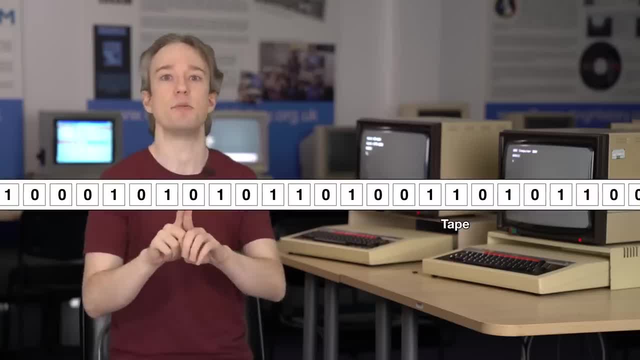 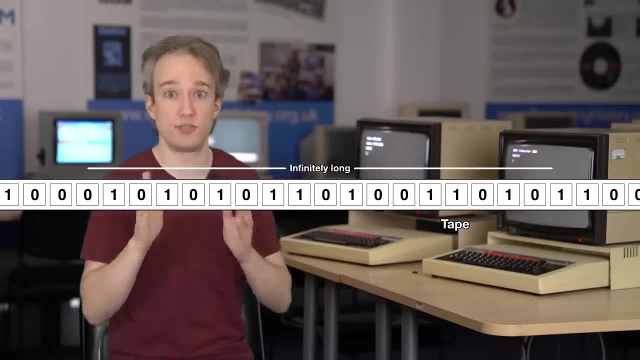 A Turing machine would be made of first a tape, And this tape would be, thanks to this existing in magical hypothetical philosophy, land, infinitely long and divided into cells. In modern terms, that's computer memory. Next, a read-write head which can move left or right over that tape. 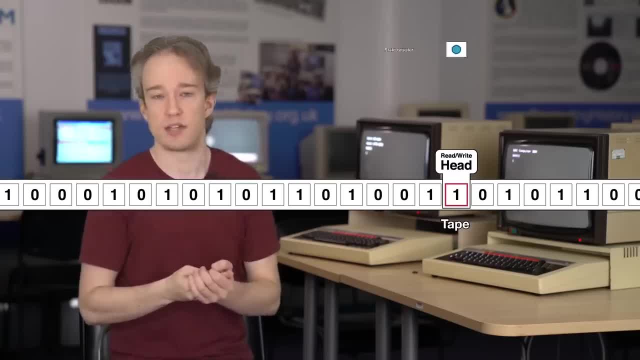 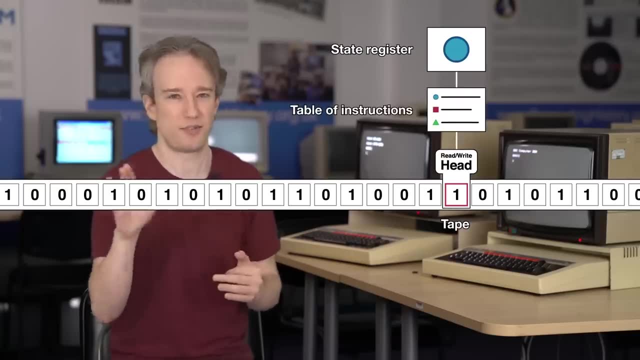 reading what's there or changing it. Then it has a state register and a table of instructions which, in modern terms, are the code. There's a lot of complicated stuff. I'm glossing over there about how this all works, but in short, it's some code. 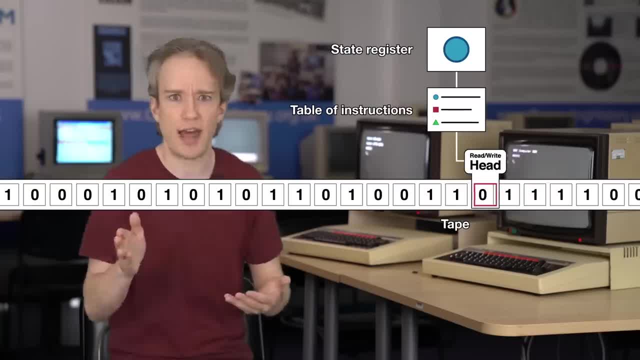 The machine follows that code, which might include instructions like: move left, move right, change what's on this bit of tape. read what's on this bit of tape and which instructions are used can depend on what those bits of tape say. Eventually, 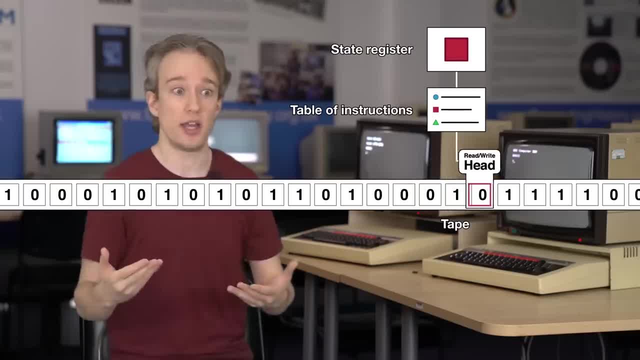 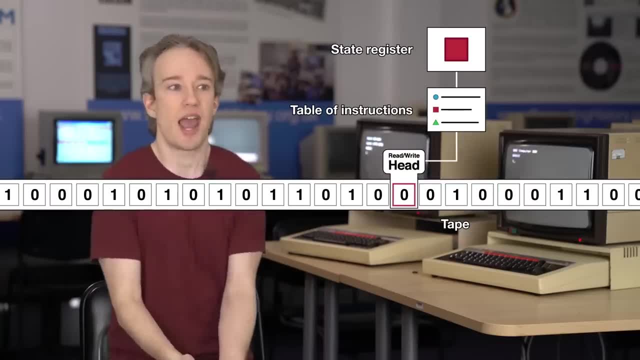 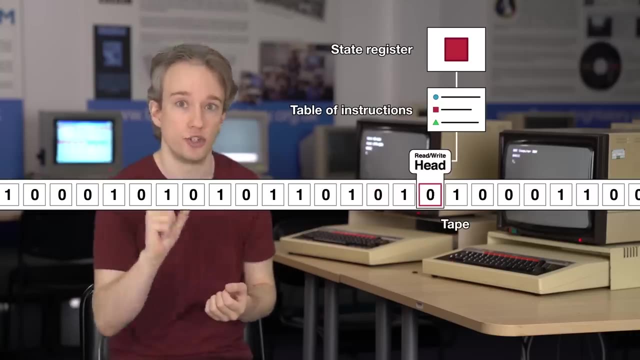 the Turing machine reaches the end of its instructions and it halts or it enters an endless loop. It was basically the minimum possible computer, but it turns out it's also every computer. Any program you write in any programming language can be converted into something that can run on a Turing machine. 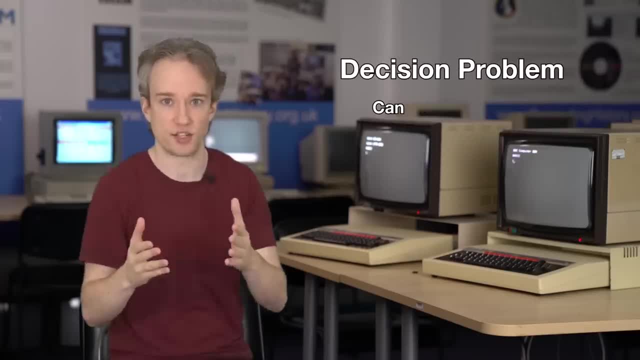 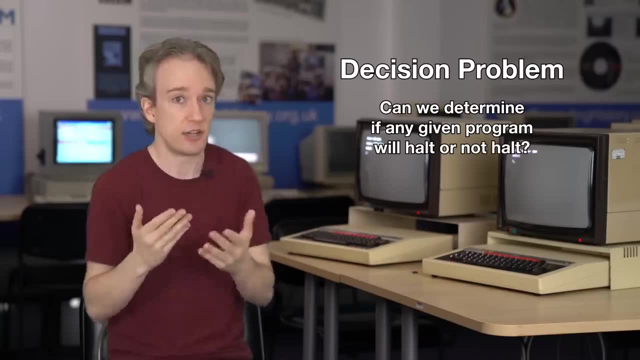 So, using that machine, Turing restated the decision problem: Can we determine if any given program will halt or not halt? Same question phrased differently. Will the machine find a solution, prove a statement, or will it keep running forever? Remember the big question that we're trying to? 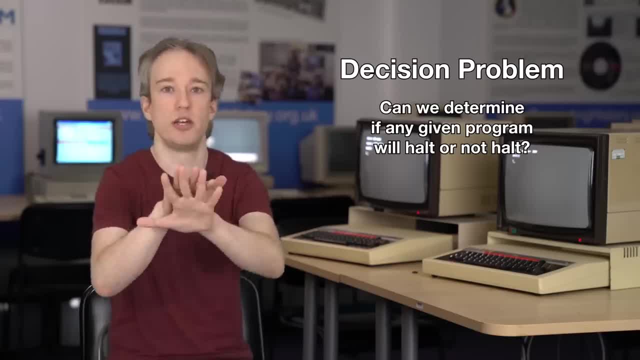 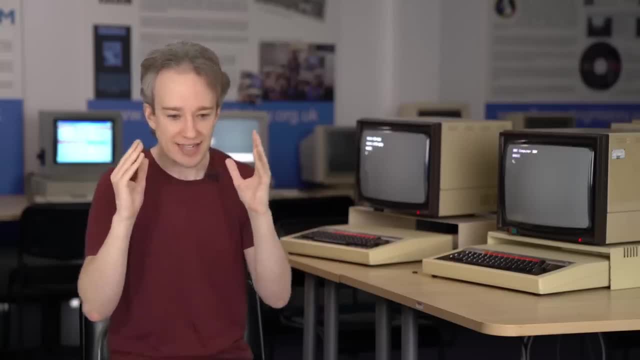 answer is: is there any question that a computer cannot solve? So Turing proposed a series of steps- and yes, I know computer scientists watching. this is a deliberate simplification. I know there are lots of subtle things I'm skipping over, but Turing 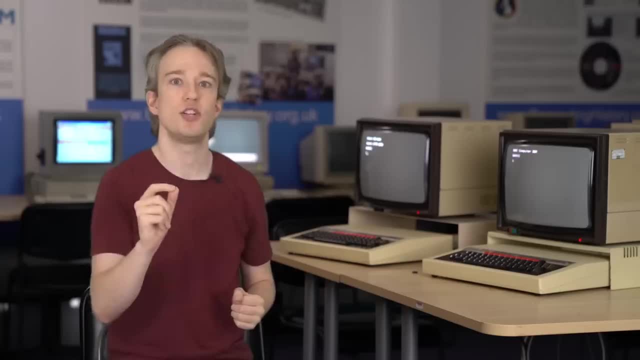 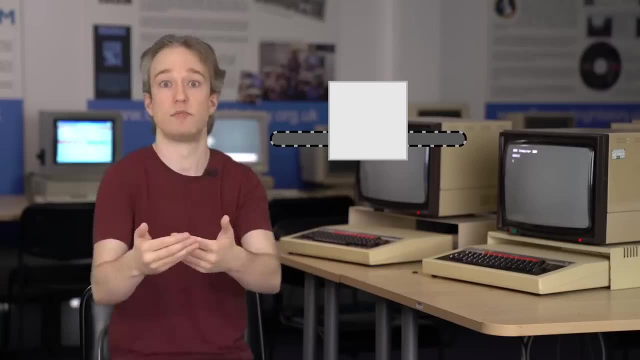 proposed a series of steps. First, imagine that we come up with a Turing machine, a program that can look at some code and figure out if that program will halt. At this point we don't need to know how that machine actually does it. 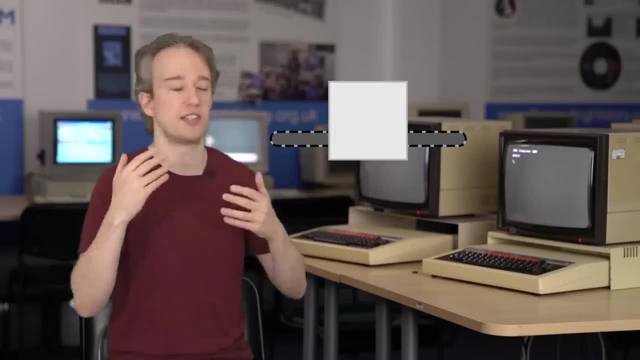 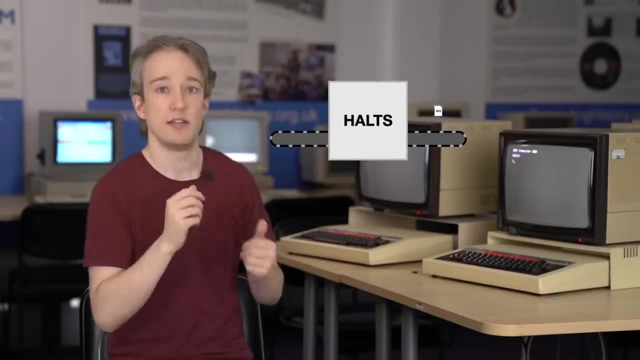 let's just assume that it works somehow. Let's call this program HALTS. HALTS takes the code for a program as its input and it outputs one of two answers: Yes, that program halts, or no, it loops forever. 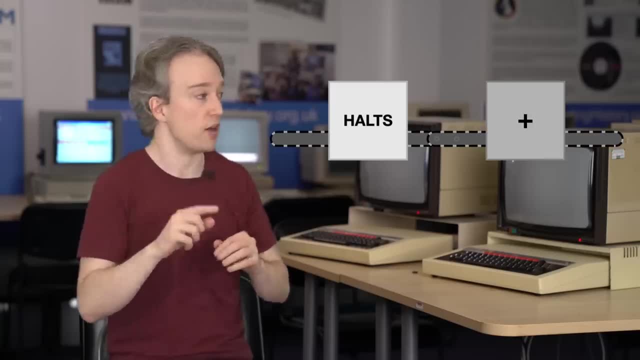 So far, so good, right, So we're going to bolt another machine, another program on the end of HALTS and, depending on the output from HALTS, it will do one of two things. If HALTS outputs, yes, knowing that the program you fed in, eventually, 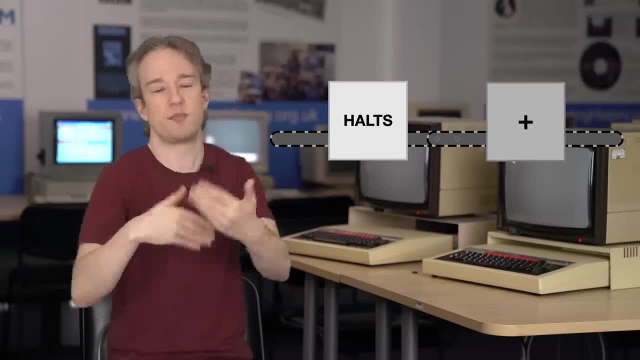 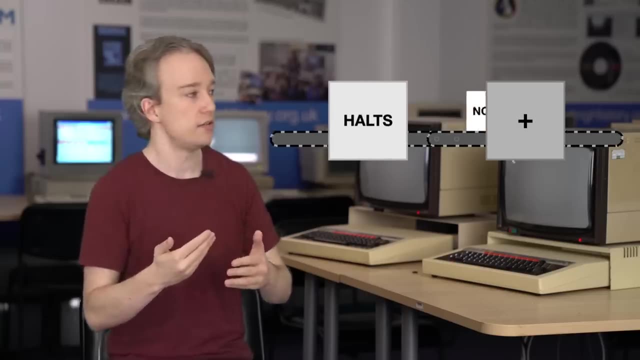 will stop, then that machine goes into an infinite loop. maybe it just prints something rude over and over whatever. And if HALTS outputs a no, if HALTS works out that the code we fed in would loop forever, then this new machine just 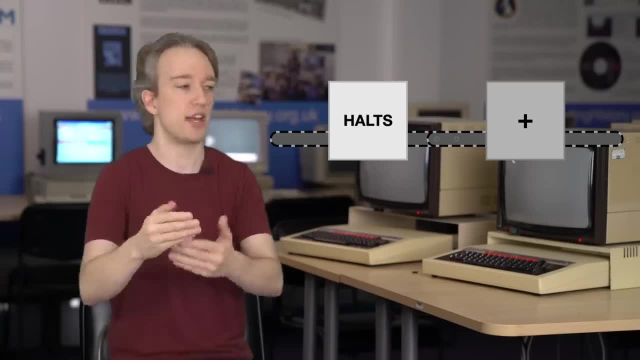 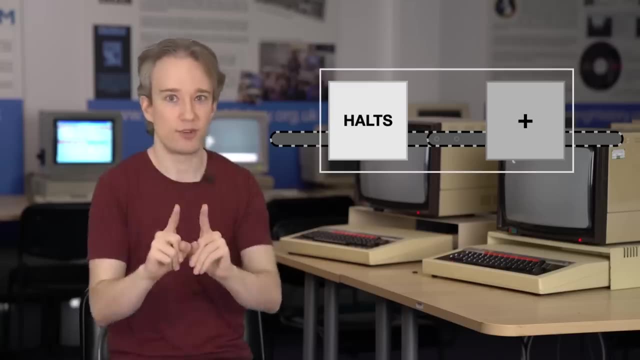 halts, OK. so if HALTS reads the code and says that'll halt, then the new machine loops. If HALTS as a program will loop, the new machine halts. We will put a box around both of those and call this whole. 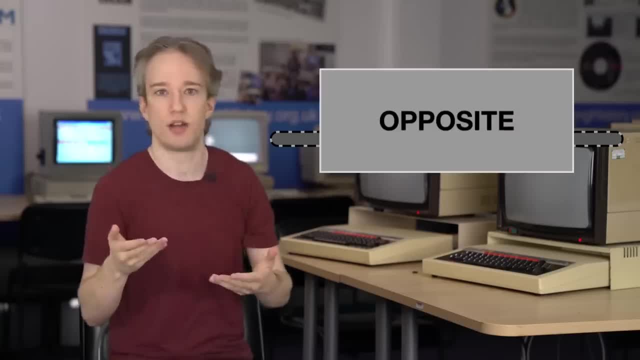 new machine. opposite, because it does the opposite of whatever code you feed it With all that set up. here's where Turing springs the trap. He proposes that we take this new combined program, our opposite. we take its code and we feed its own code into itself. 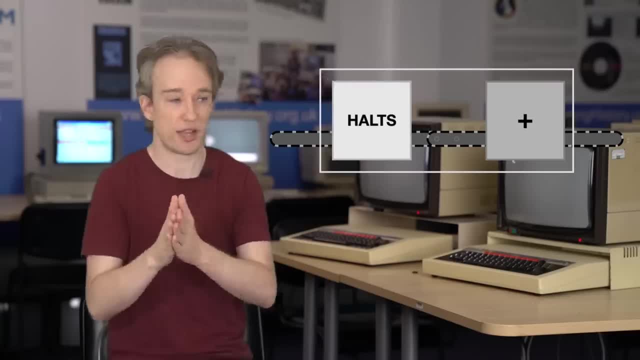 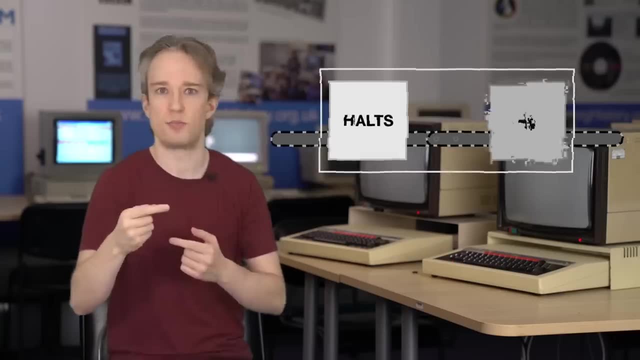 What will it do? Well, let's step through the logic. If it thinks the answer is this code will halt, then it will loop. But then the answer is: it'll loop, so it'll halt, but then it'll halt, so it'll loop, but then it'll. 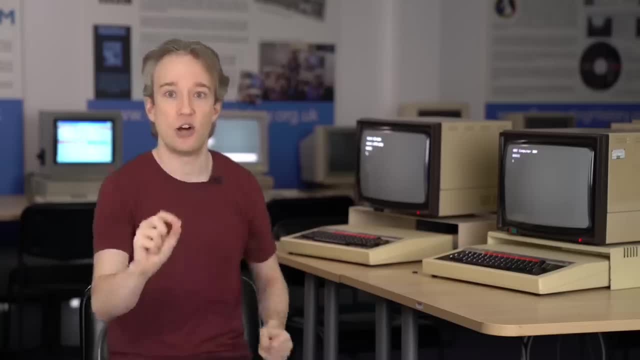 and it vanishes in a puff of logic. To be clear, that's not a loop in itself, that's a paradox, that's a logical, mathematical impossibility. and that is Turing's answer to the decision problem. If you ever have a program that can determine for certain. 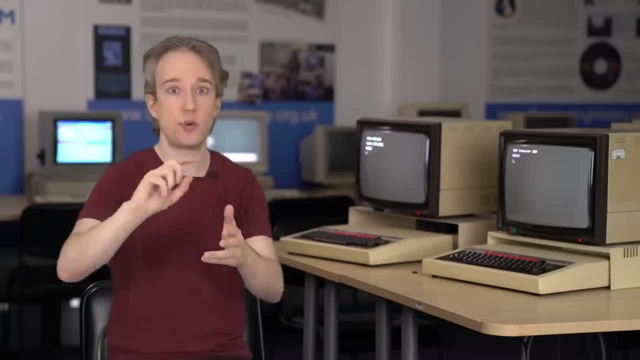 whether any particular program will halt or loop. you can easily tweak it a little, let it contradict itself and cause that paradox, And that's impossible. So a program to do that can not exist, Which means there's definitely an exception. There is definitely at least one thing that computers cannot: 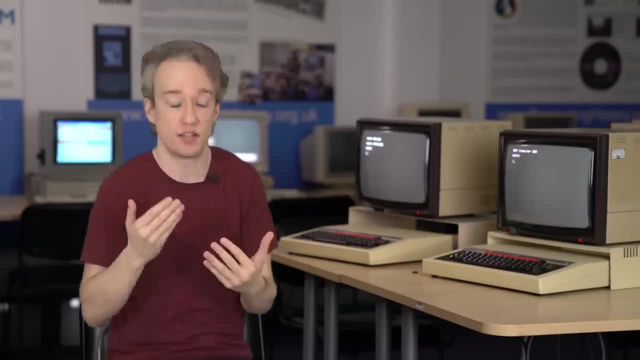 ever solve, even given infinite time and power, The answer to the decision problem. the answer to the question: can we determine if every program will halt or not? halt, no, Now there are obviously a lot of programs where you can easily tell at a glance if they'll halt or not. 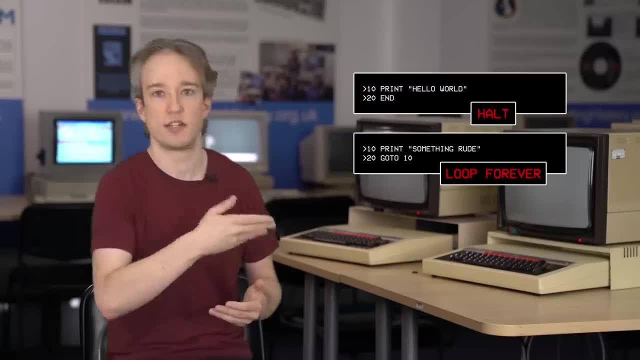 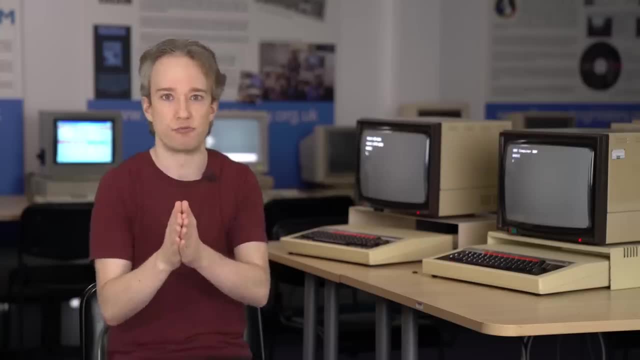 this code will loop forever. That code will exit and halt. The decision problem isn't about whether you can tell if some programs will halt or loop. That's easy. It's about every program. It's about the fundamental fact that there are definitely some things.